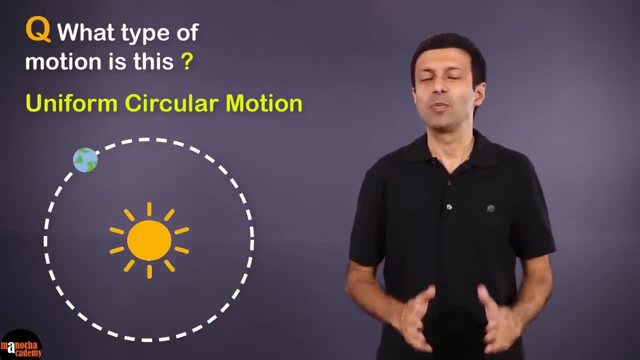 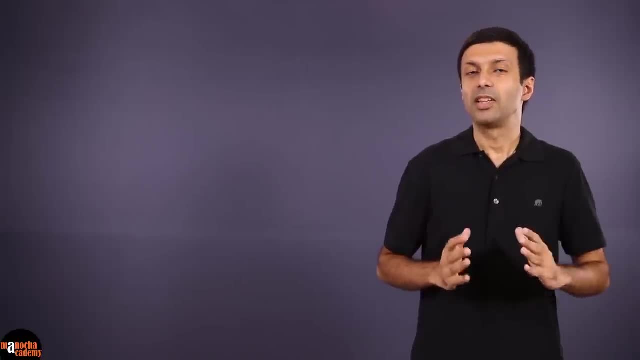 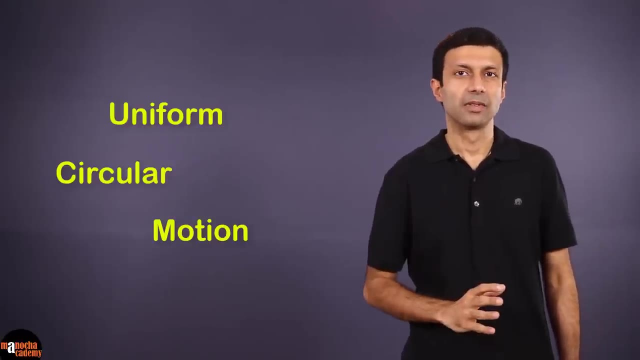 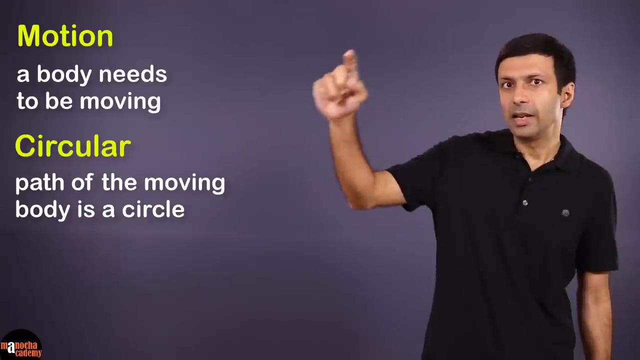 I am sure by the end of the video the concepts are going to be super clear to you. To understand the term uniform circular motion, let's break it down. There are three words here: uniform, circular and motion. Let's start from the back. Motion means a body needs to be moving, Circular means the path of the moving body has the shape of a circle, And uniform means the body is moving at. 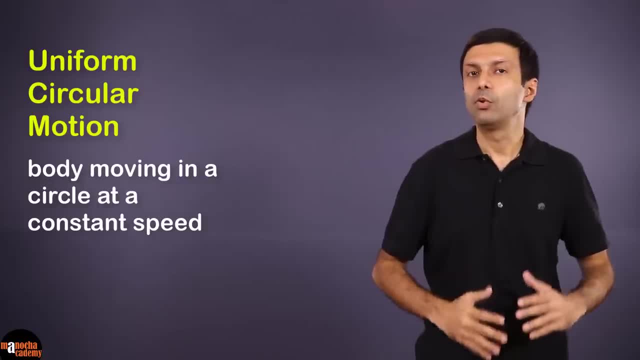 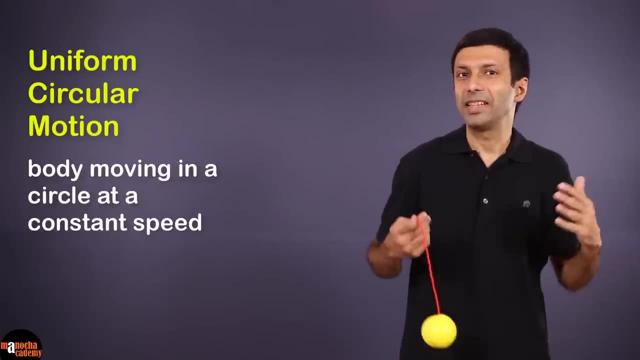 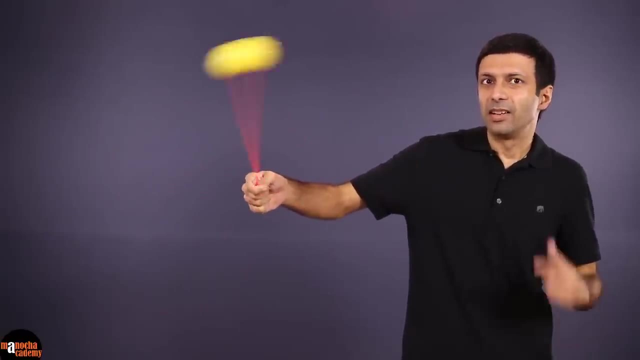 a constant speed. So a body moving in a circle at a constant speed is known as uniform circular motion. Now let's apply this definition of uniform circular motion to our ball example. So, as you can see, the ball is moving and it's moving in a circle. The ball is moving at a constant speed, which means it's moving at the same pace. It's not going faster, it's not going faster. 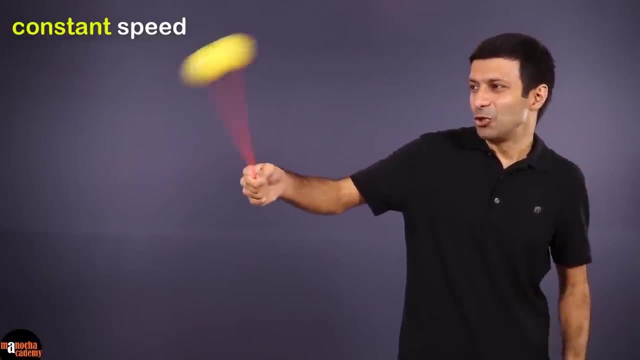 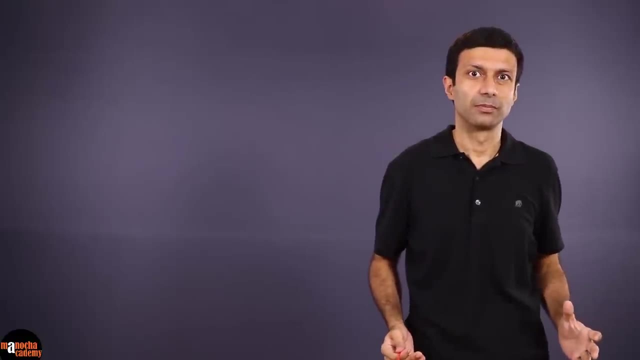 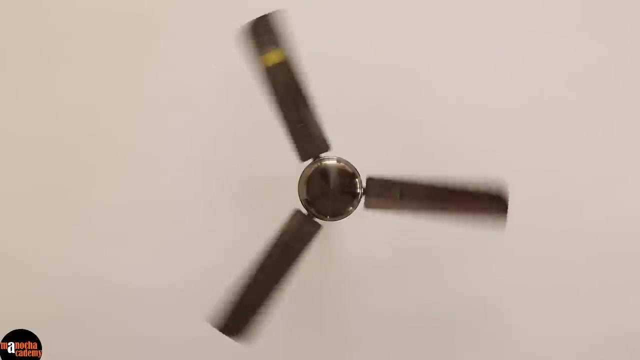 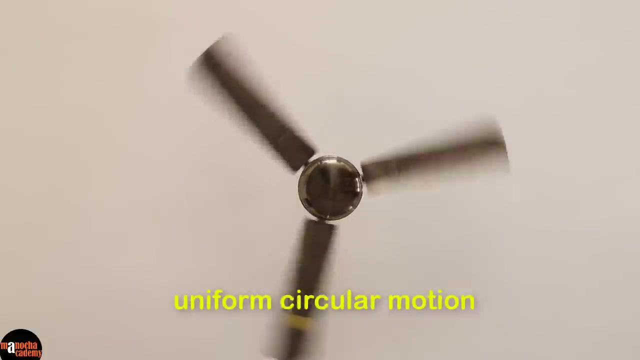 Or slower. Of course, it's hard for me to keep it at a constant speed, And that's why the fan is a better example of uniform circular motion. So when you switch on the fan and give the fan some time to reach its fixed speed. Now, if you consider this sticker on the fan blade, can you see it's in uniform circular motion, It's moving in a circle at a fixed speed. How do we calculate the speed? 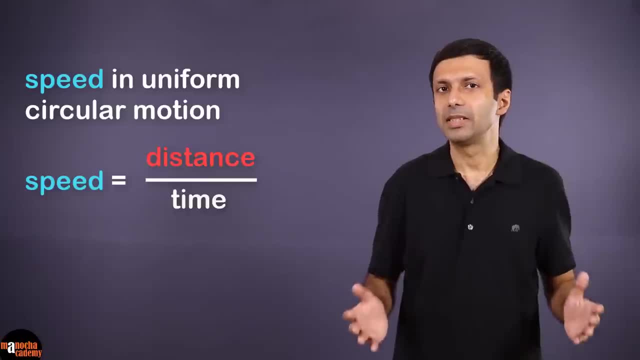 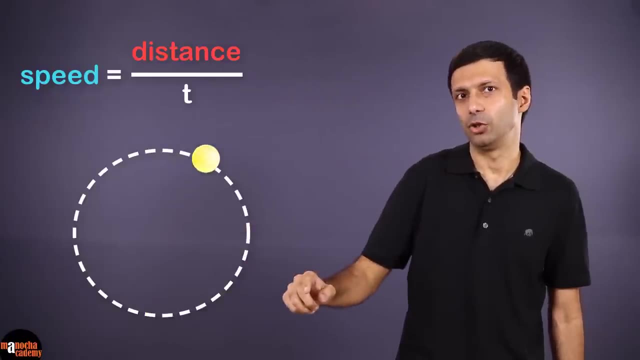 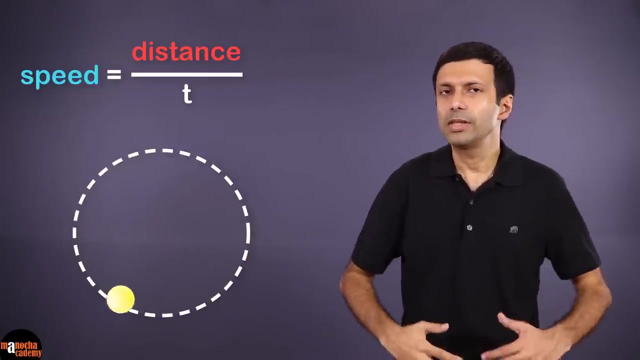 In uniform circular motion. We know that speed is distance by time. Let's say the body takes t seconds to complete one full revolution. So that's t seconds to complete one full circle. Now what is the distance traveled here? That's right, It's the circumference of the circle. So that's 2 pi r, where r is the radius of the circle. 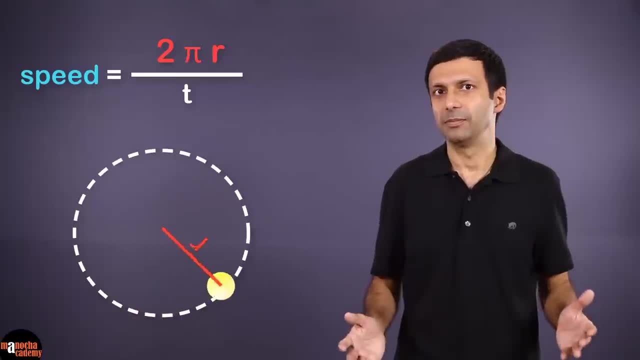 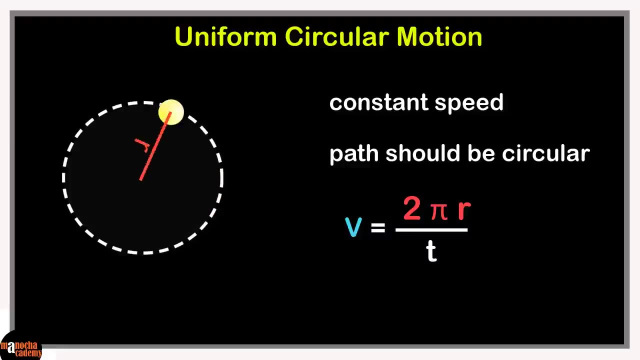 So the speed of the body is 2 pi r by t, Or we say that the magnitude of the velocity is 2 pi r by t. Let's place the concept of uniform circular motion and the formula to calculate its velocity on our concept board. 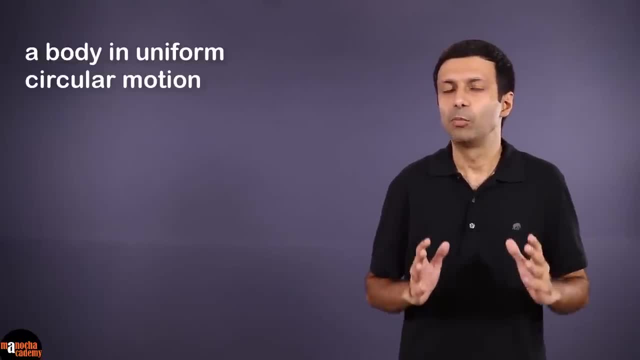 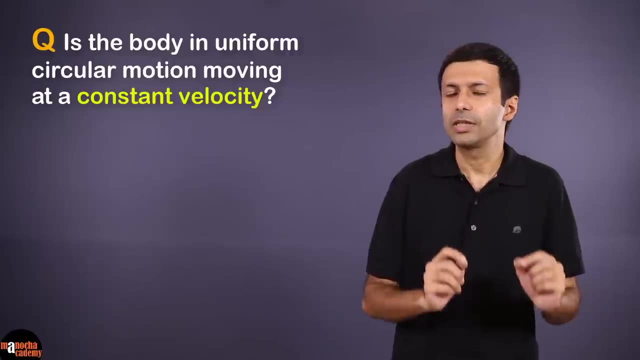 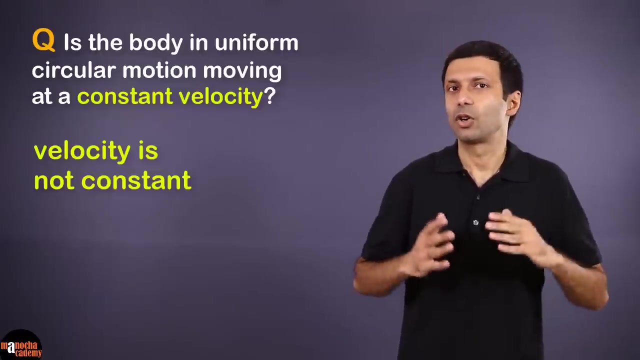 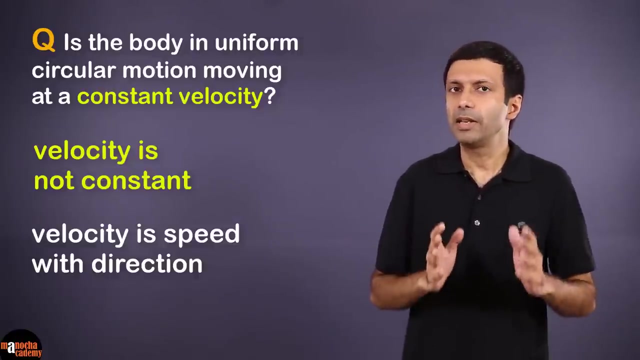 We know that a body in uniform circular motion is moving at a constant speed. Now an interesting question is: is the body also moving at a constant velocity? What do you think That's right? The velocity is not constant. Remember, velocity is speed with direction. So the speed here is constant, But is the direction also constant? 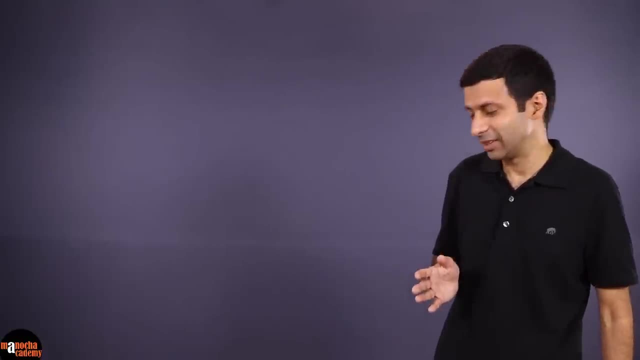 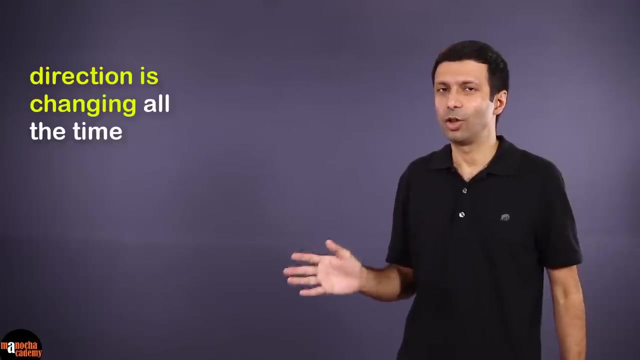 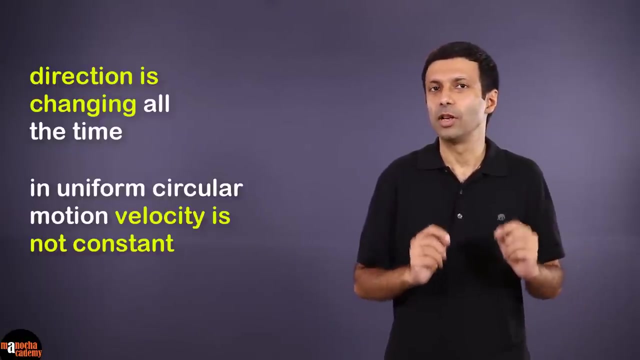 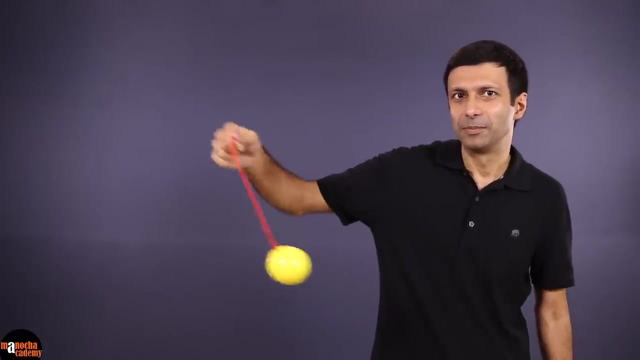 Why don't you try walking around the room in a circle like this? Can you feel that your direction is changing all the time? So if the direction is changing, velocity is also changing. So in uniform circular motion, velocity is not constant. Let's consider the ball and rope example. Now, what is the direction of the velocity of the ball at any instant? 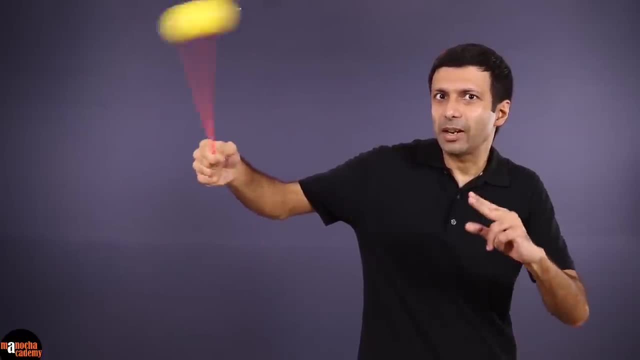 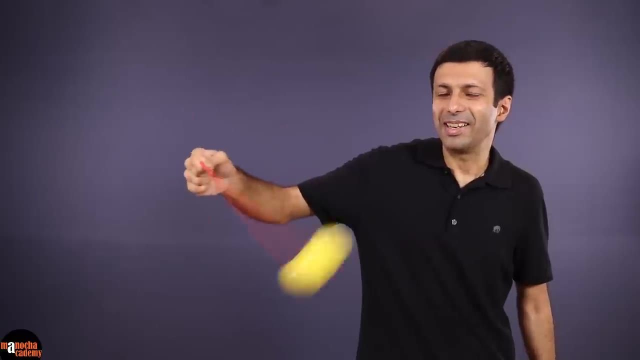 To visualize. you can imagine that we cut the rope. Or if I leave the rope, in which direction will the ball go? So let's go ahead and try it. I am going to leave the rope and you carefully look which direction the ball is going to go. 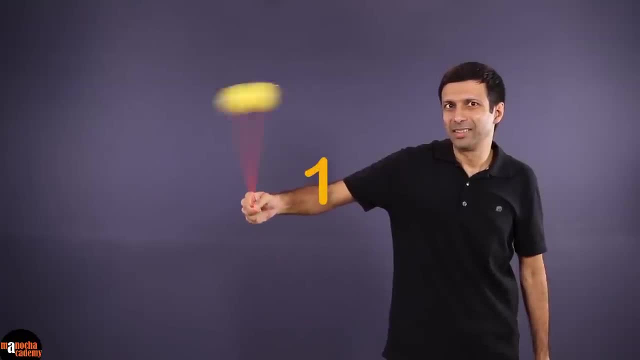 Are you ready? One, two, three. Now let's take a look at the slow motion replay. In the slow motion replay, can you see that the ball goes off in a straight line when I leave the rope? If you draw the radius of the circle, at that point the direction of the velocity is perpendicular to the direction of the ball. 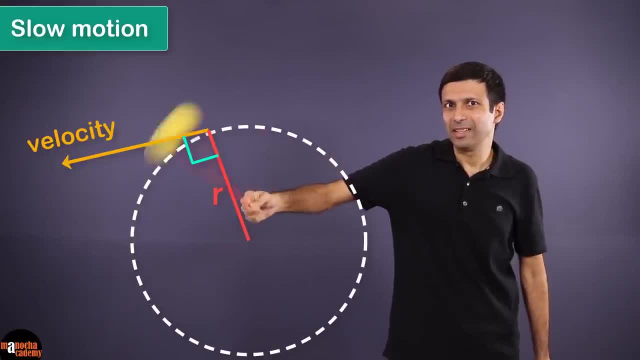 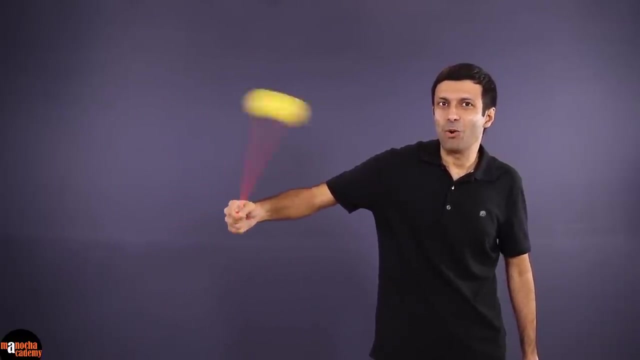 It is perpendicular to the radius of the circle, This is called a tangent to the circle at that point. That's why it is called a tangential velocity. Similarly, if I set the ball into uniform circular motion again and now I leave it at a different place, 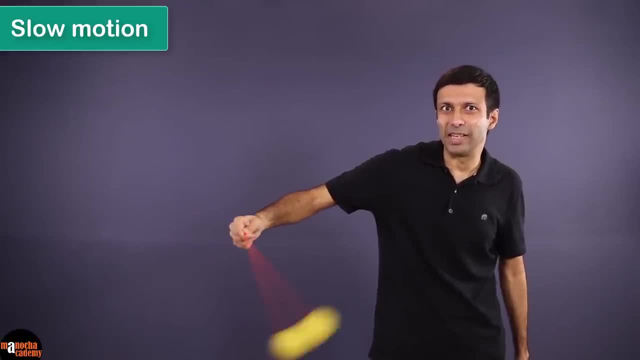 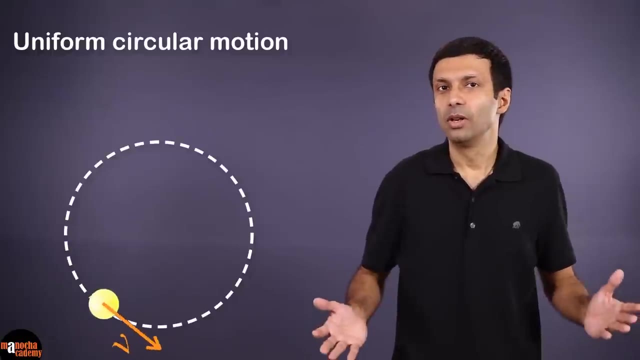 If we look at the slow motion replay, can you see that the ball flies off in a straight line. That is a tangent to the circle. at that point Now we know that a body in uniform circular motion is moving in a circle at a constant speed. 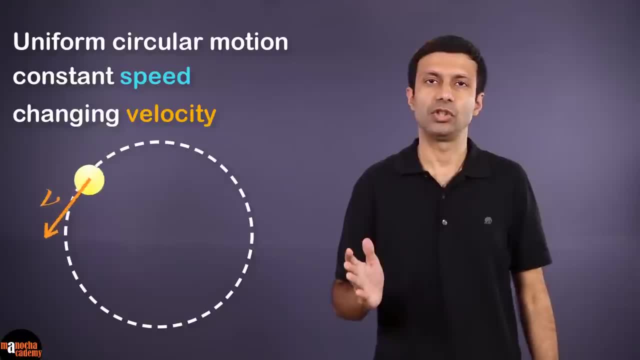 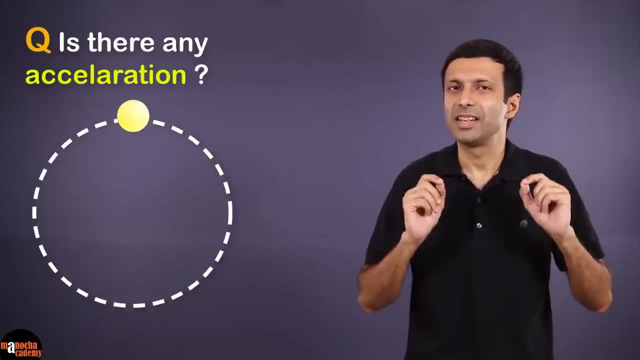 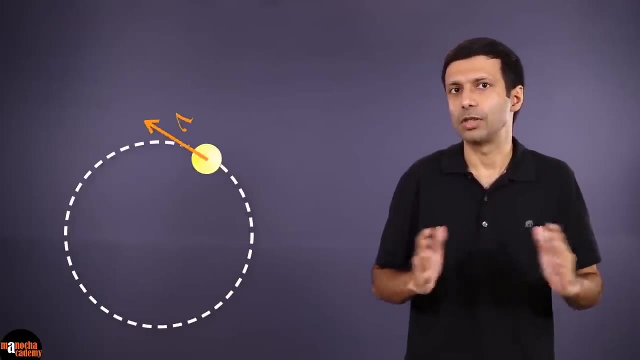 but changing velocity because the direction is changing. An interesting question is: is there any acceleration? here The answer is yes, It's an accelerated motion. Now, if you look only at the speed, the speed is constant, So it looks like there is no acceleration. 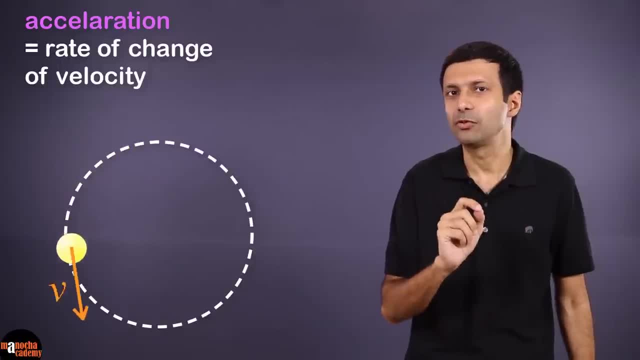 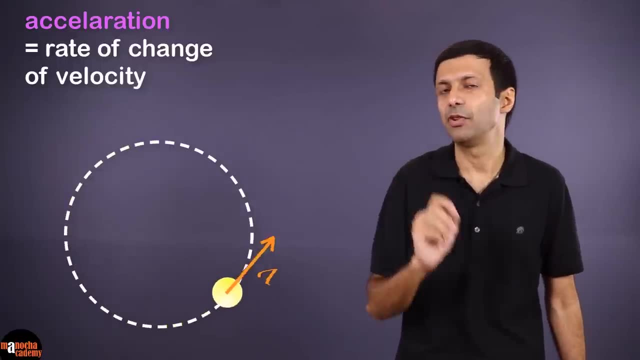 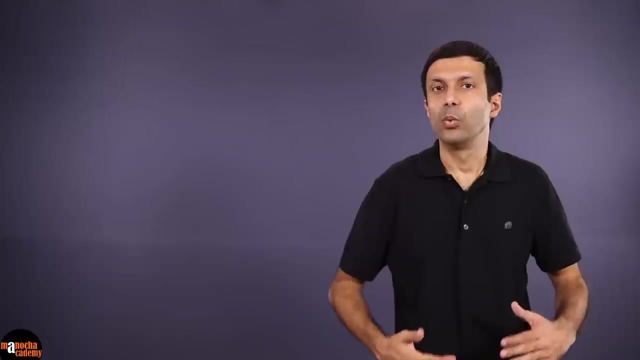 But remember, acceleration is the rate of change of velocity. The magnitude of velocity may be same, but the direction is definitely changing, as we saw. So this is clearly an accelerated motion. We know that the direction of the velocity is along a tangent to the circle. 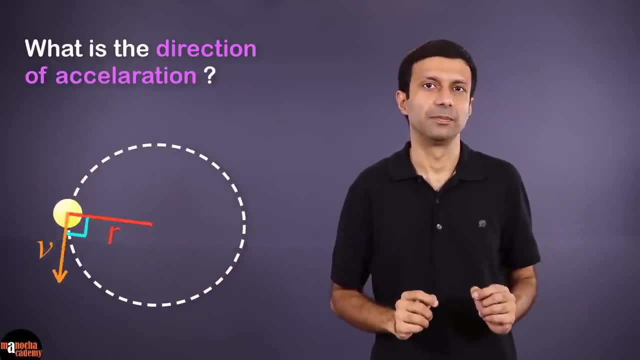 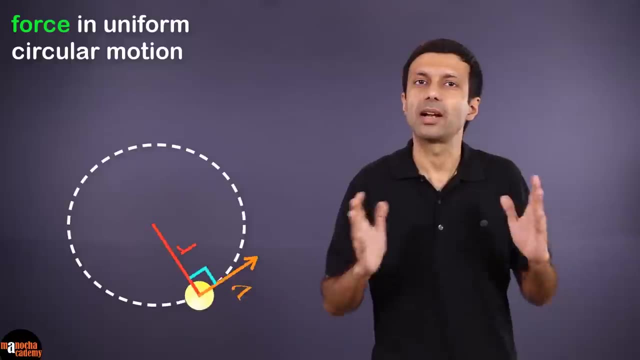 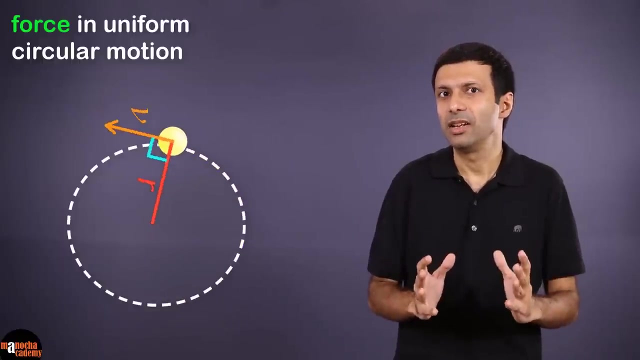 But what is the direction of the acceleration? Now, that's a little more tricky. So, to simplify, first we'll look at the force and then we'll come back to the direction of acceleration, Since in uniform circular motion there is an acceleration. 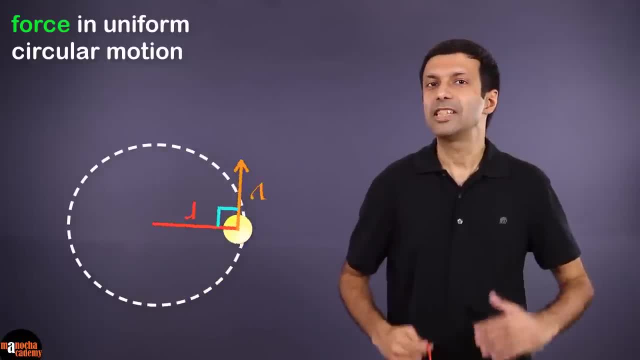 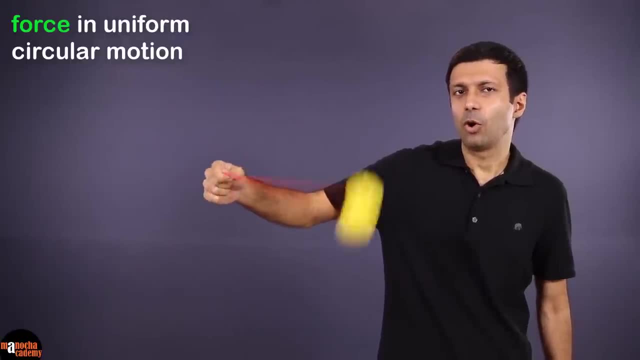 there must be some force involved. Let's look at the force in uniform circular motion. So try swinging the ball around like this. Or maybe for the force. I think it might be easier to visualize if you swing the ball around like this. So where is the force here? 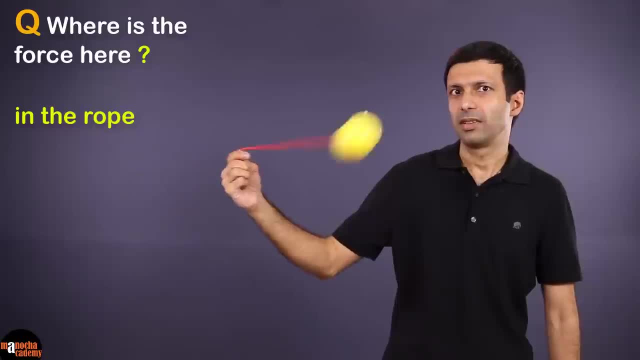 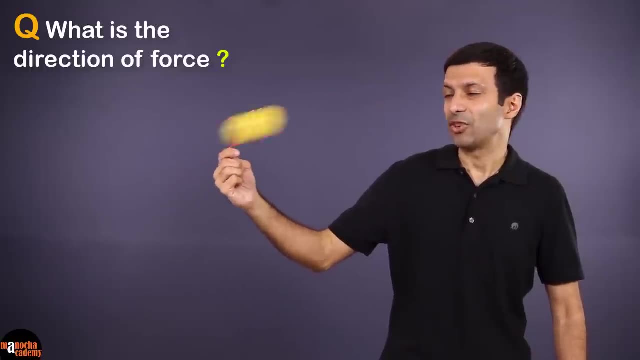 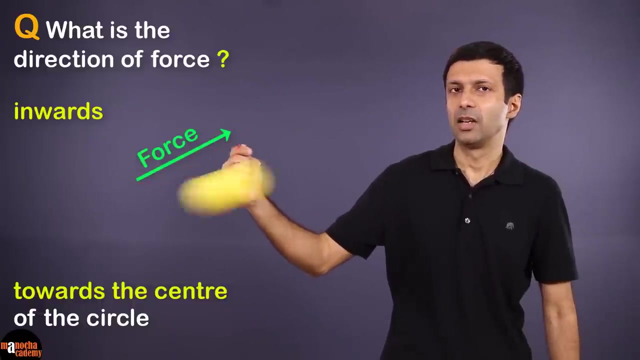 That's right, it's in the rope. It's the tension in the rope here. Now, what is the direction of the force? That's right, it's inwards, towards the center of the circle, which is my hand here. So my hand is continuously pulling the ball with the rope towards the center. 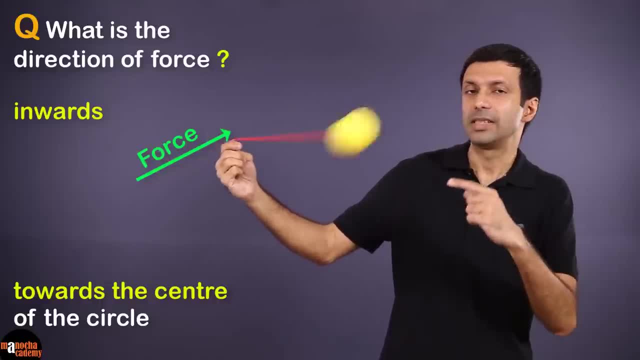 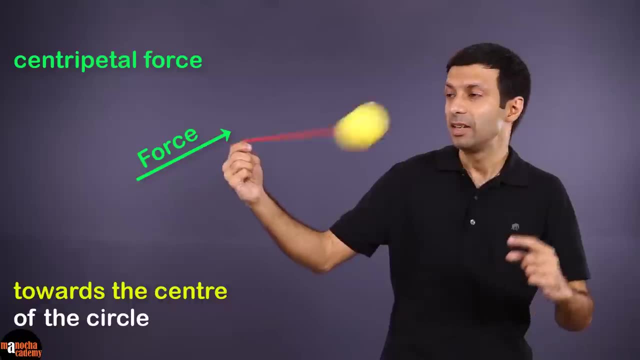 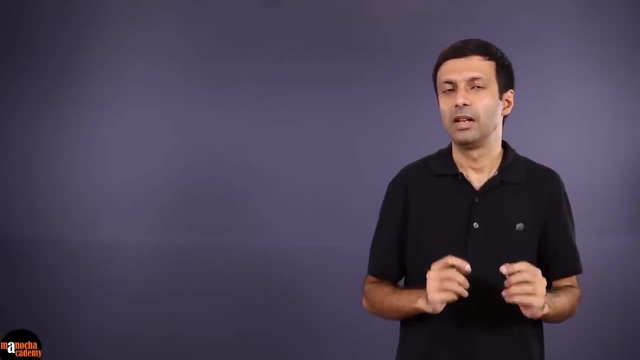 And the direction of the force is continuously towards the center of the circle. This is known as centripetal force, because the word centripetal means center-seeking. Similarly, if you consider the Sun and Earth example, the Sun's gravitational force is keeping the Earth in uniform circular motion. 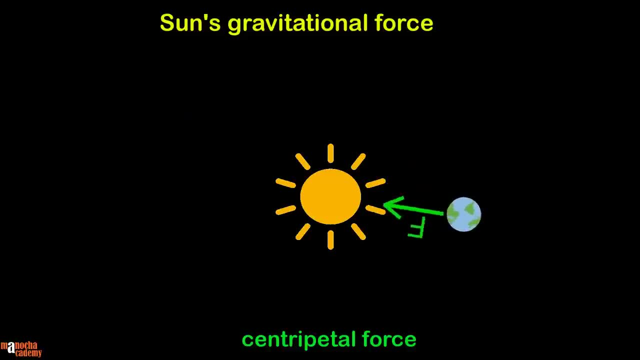 The gravitational force is a centripetal force, That is, it's a center-seeking force. It's continuously pulling the Earth towards the center of the orbit, which is the Sun in this case. Now, for example, let's say, today is Sunday. 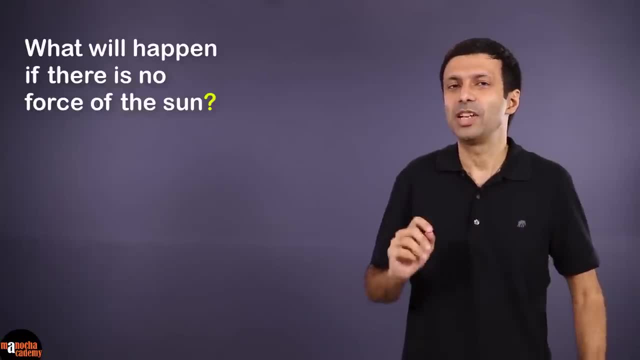 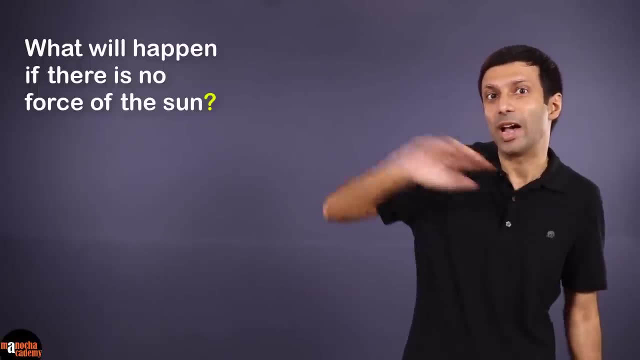 and the Sun says: I'm tired, I need a break. So there's no force on the Earth. What do you think is going to happen? That's right, the Earth is going to fly off into space, just like the ball. when I left the rope. 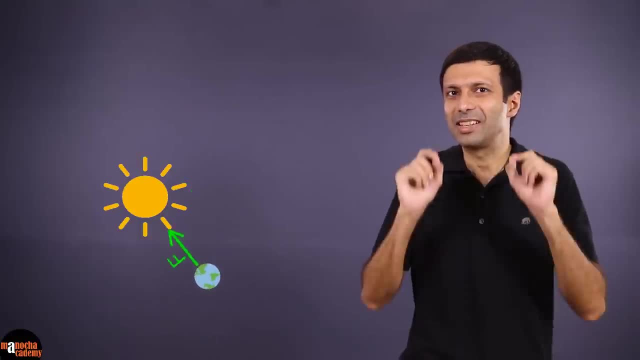 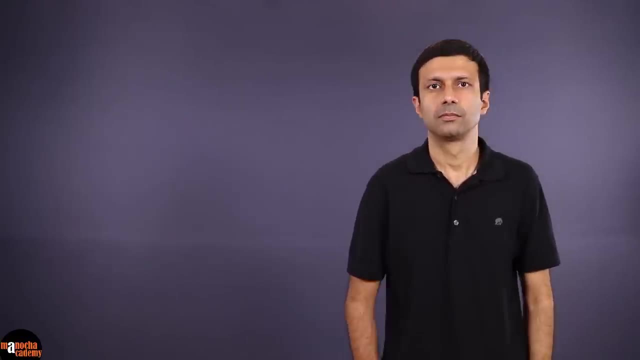 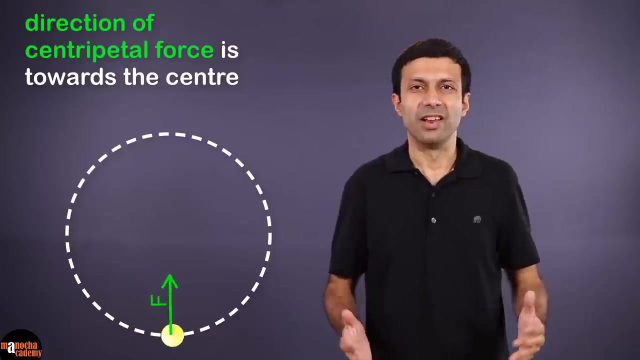 So thankfully the Sun never takes a holiday, because this centripetal force is necessary to keep a body in uniform circular motion. We know that the direction of the force is towards the center. It's a centripetal force. Now the direction of the acceleration is easy. 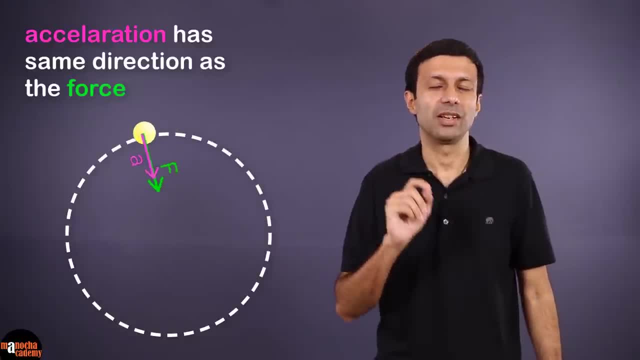 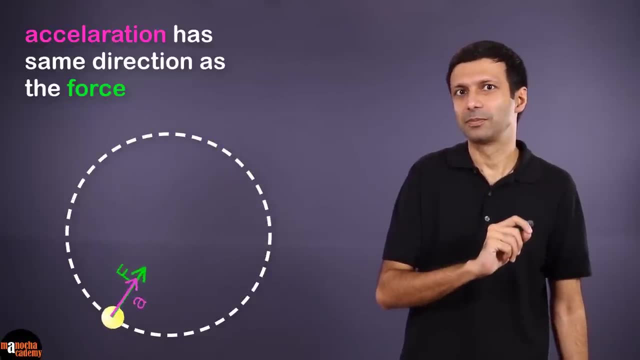 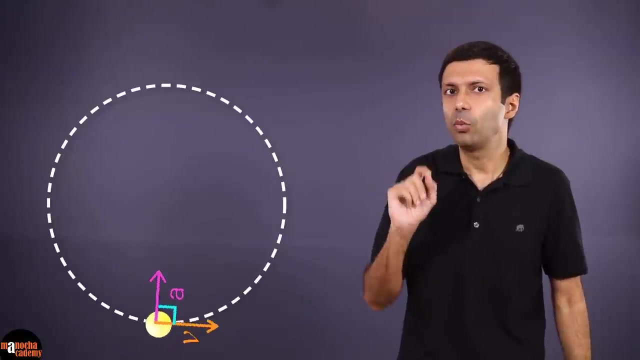 because acceleration has the same direction as the force, So the direction of the acceleration is also towards the center of the circle. So this is called a centripetal acceleration, And the direction of the acceleration is always perpendicular to the direction of the velocity at that instant. 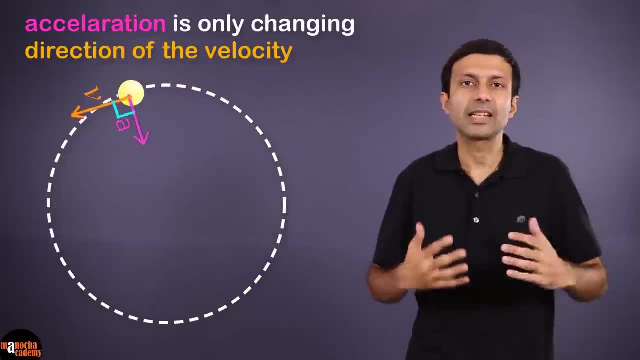 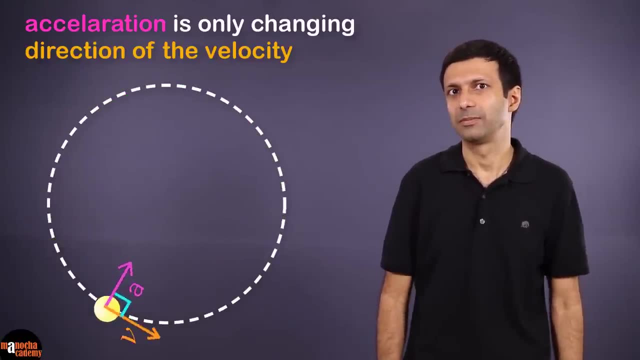 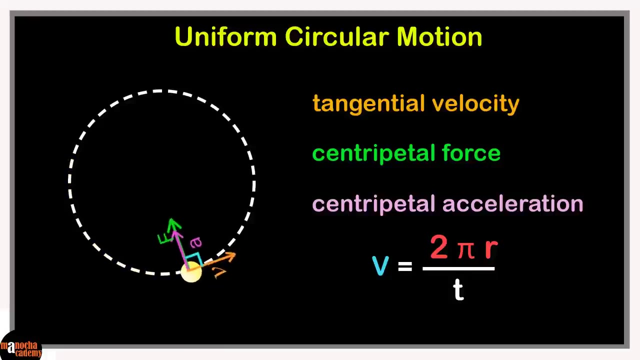 as shown here, And the acceleration is only changing the direction of the velocity, not the magnitude of the velocity. Let's put the concepts of velocity, acceleration and centripetal force for uniform circular motion on our concept board. I hope the concept of uniform circular motion. 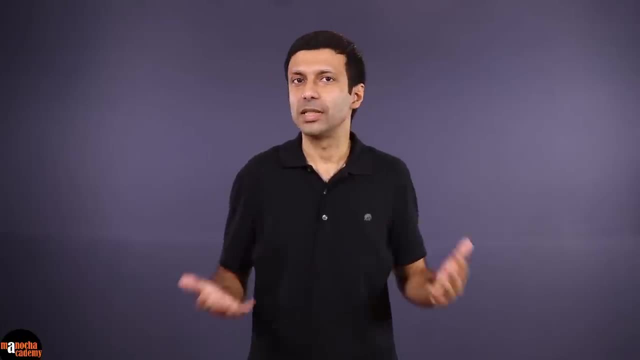 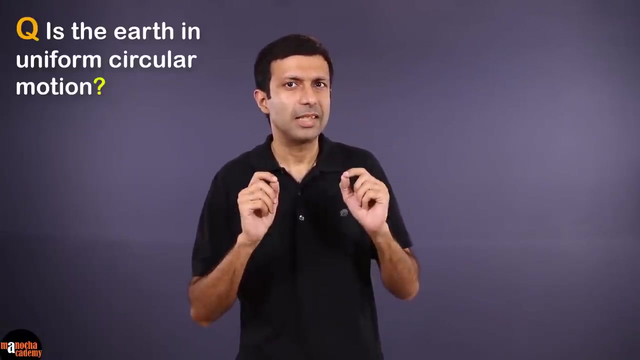 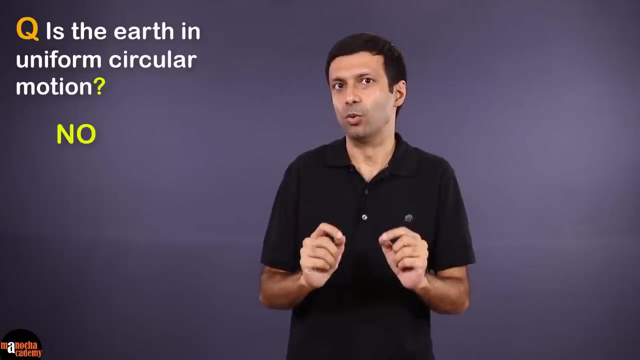 is crystal clear to you now, As we discussed: the Earth going around the Sun is an example of uniform circular motion. But is this really true? Your textbooks may also say that, but the correct answer is no, Because, strictly speaking, the Earth is not in a uniform circular motion. 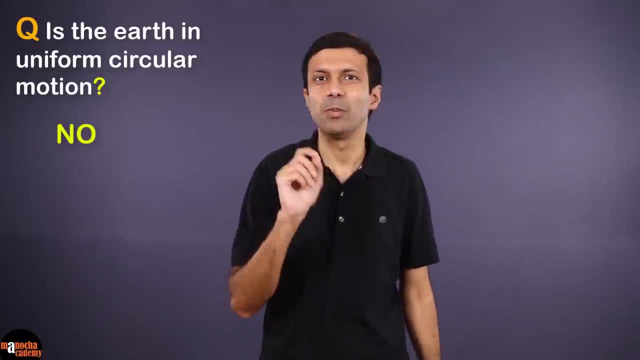 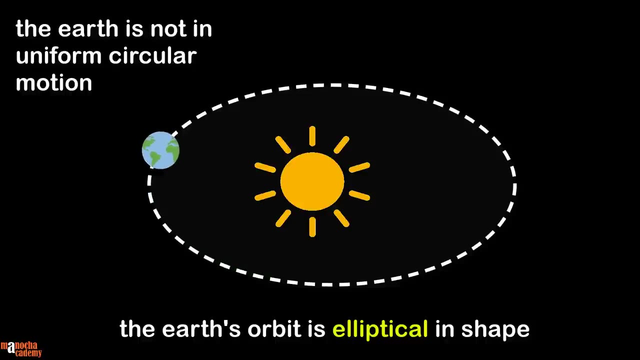 Now, why is that? Because, as you may know, the Earth's orbit is not perfectly circular. It's elliptical in shape, And you know that the Earth, when it's closer to the Sun, is moving much faster than when it's away from the Sun. 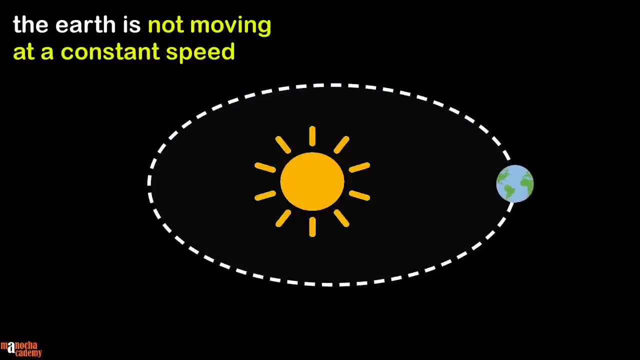 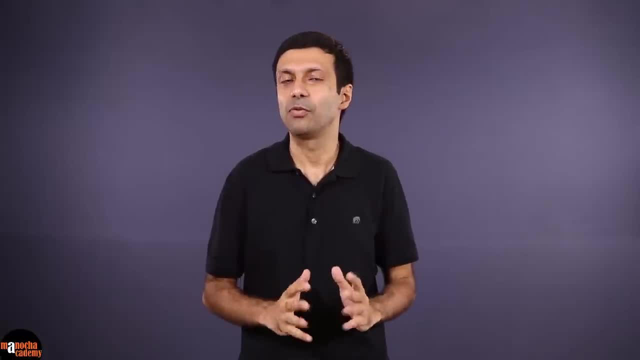 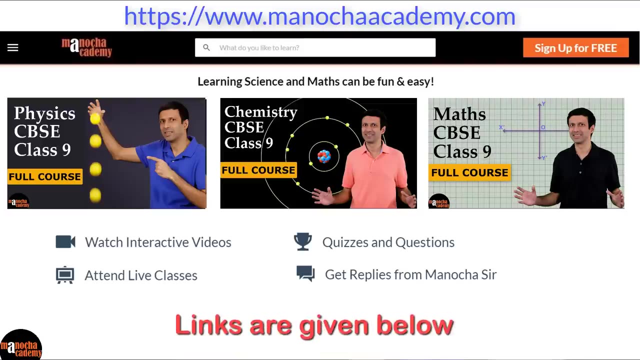 So the Earth is not moving at a constant speed. But usually we ignore all these details and we consider Earth moving around the Sun as an example of uniform circular motion. So this is an approximation that we make To watch more science and maths videos like this.